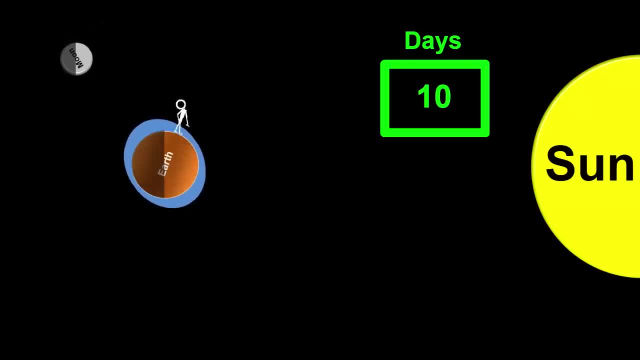 After another seven days or so, the Moon orbits to the opposite side of the Earth, to the Sun, and we can see that the Sun is moving towards the Moon And we can see its full day side. This is the full Moon. Then it continues onto the third quarter. 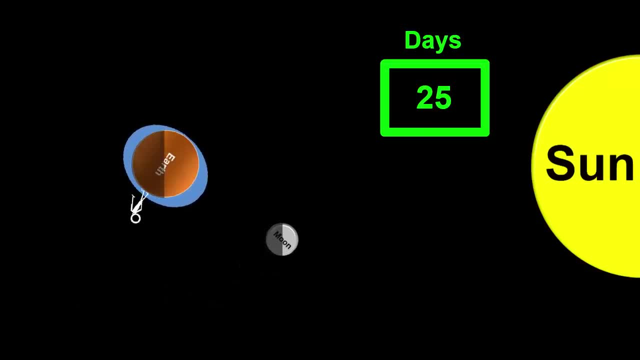 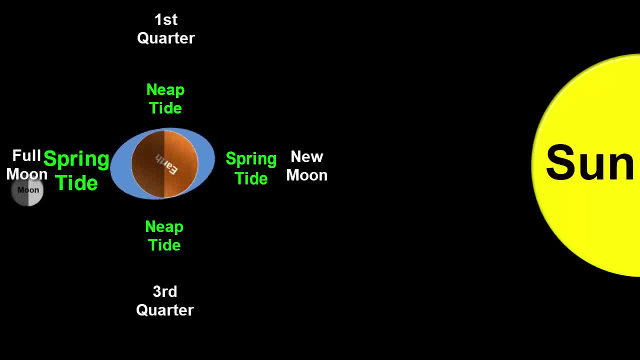 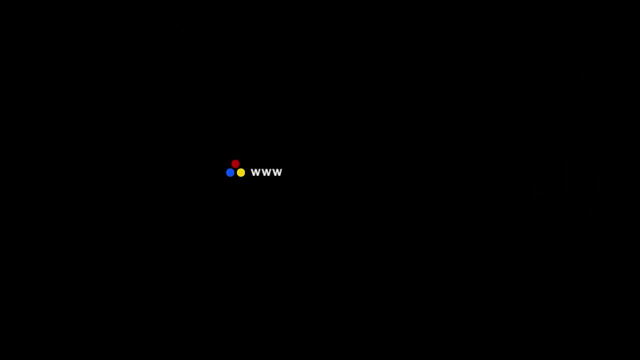 But this is important. when the Sun and Moon line up, so their gravitational attractions combine to make supertides. But this is important. when the Sun and Moon line up, so their gravitational attractions combine to make supertides. But this is important. when the Sun and Moon line up, so their gravitational attractions combine to make supertides.